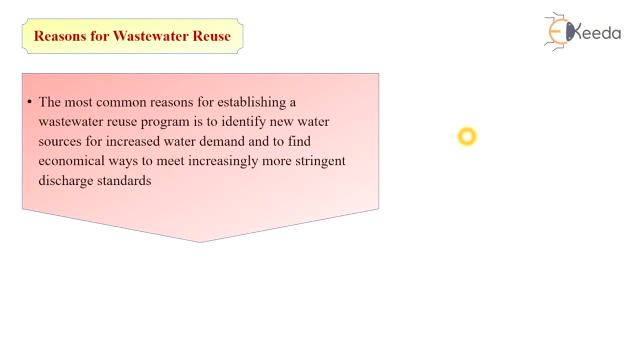 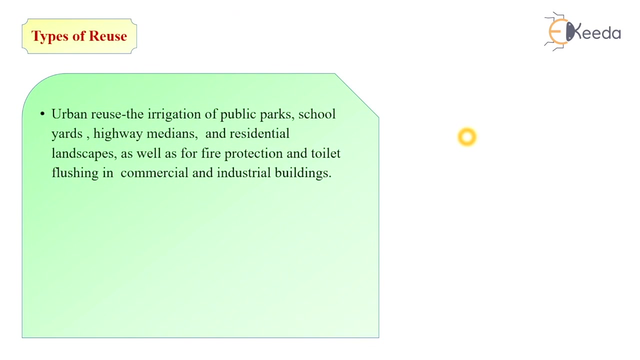 And to find the economical ways to meet increasingly more strict, more stretch and discharge standards. So nowadays, people facing the water scarcity and for increasing the water demand, we are reusing this wastewater for the different purposes, So types of reuse, In different way or in different form or in different times we are 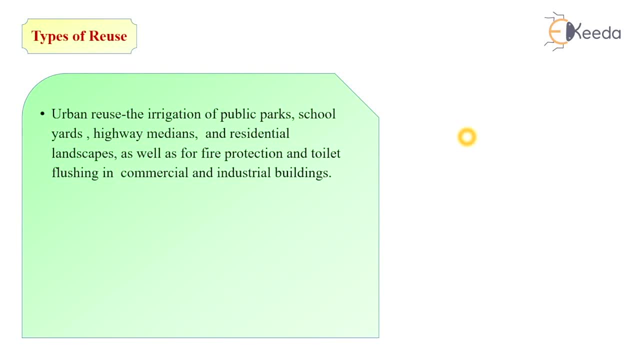 reusing the wastewater. So, for example, in urban area. So in urban reuse, while we are reusing the water in urban areas, the irrigation of public parks, schools, yards, highway medians and residential landscape, as well as for fire protection and toilet flushing in commercial and industrial buildings. 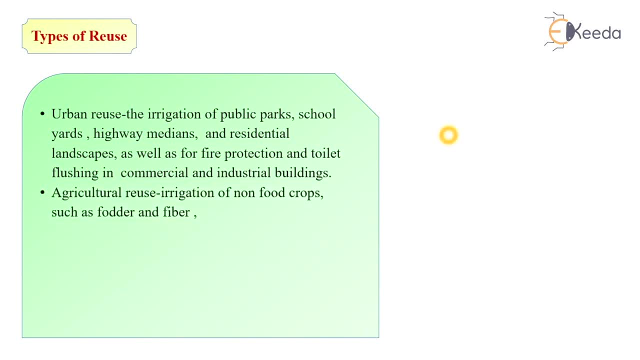 And agricultural reuse. the irrigation of non-food crops, such as fodder and fibers In commercial nurseries and pasture lands. the high-quality reclaimed water is used to irrigate the food crops, Recreational impoundments such as ponds and lakes. So, like these different functions, for carrying different functions, we are providing the 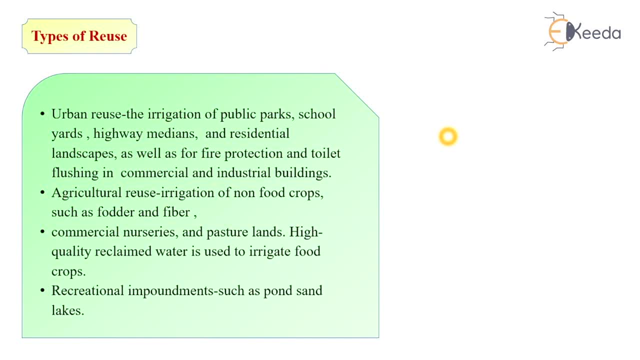 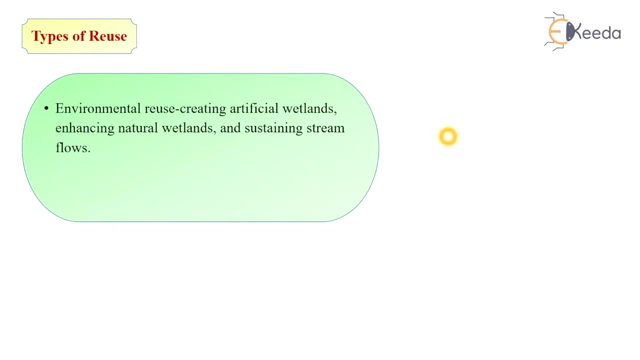 reuse water for this purposes- For irrigation purpose, for urban reuse purpose, for commercial and industrial reuse purpose, etc. Again, for the environmental reuse- creating the artificial wetland, enhancing natural wetland and sustaining steam flows- Industrial reuse process or make-up water and cooling tower water are required. 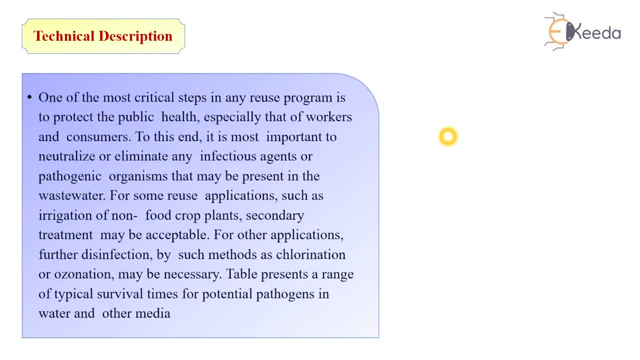 So technical descriptions How we are going to reuse this water. So one of the most critical steps in any reuse program is to use the water in a way that is suitable for the environment. So one of the most critical steps in any reuse program is to use the water in a way that is suitable for the environment. 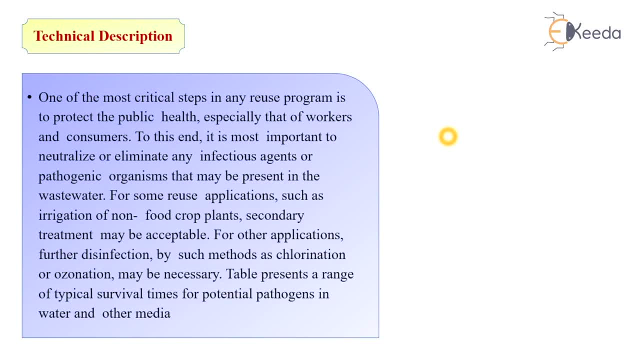 To this end, it is most important to neutralize or eliminate any infection agents or pathogenic organism that may be present in the wastewater. For some reuse applications, such as irrigation for non-food crop plants, secondary treatment may be accepted. For other applications, such as further disinfection by 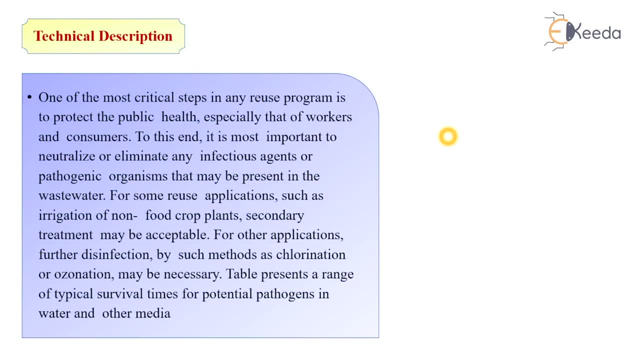 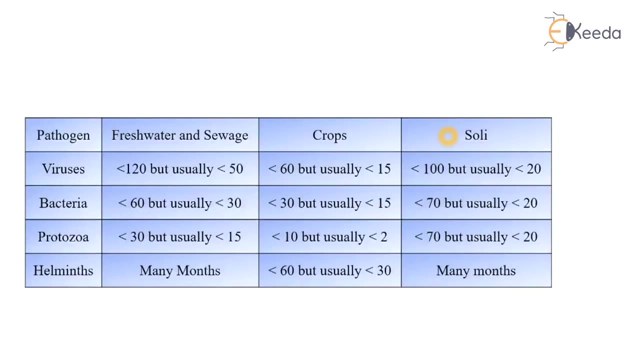 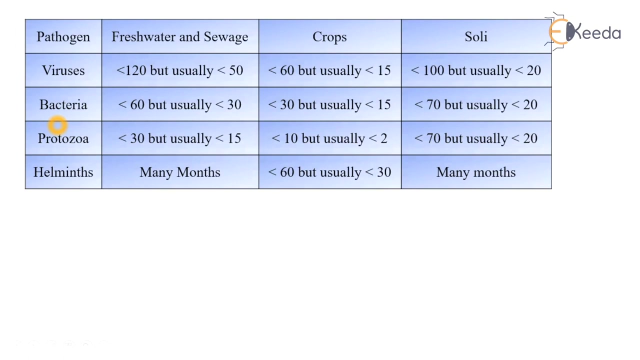 For other applications, such as further disinfection by such method as chlorination or ozonation, may be necessary. In next slides we are see the table which presents a range of typical survival time for potential pathogens in water and other mediums. So, as you can see in this chart, these are the types of some pathogens which are present. 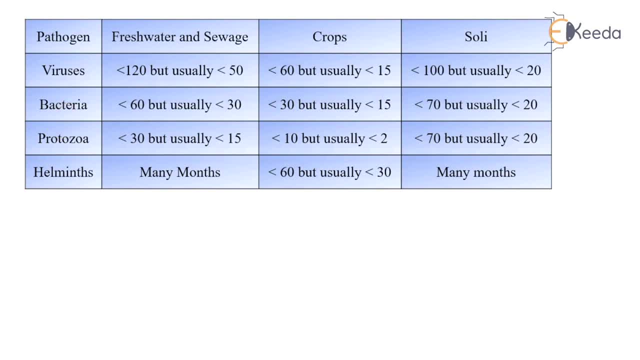 in the sewage that are viruses, bacteria, protozoa and helminths. So these are the time limits on that time these bacteria are surviving in this particular sewage or wastewater. So in freshwater and sewage the viruses are present for the duration of less than 50 minutes. 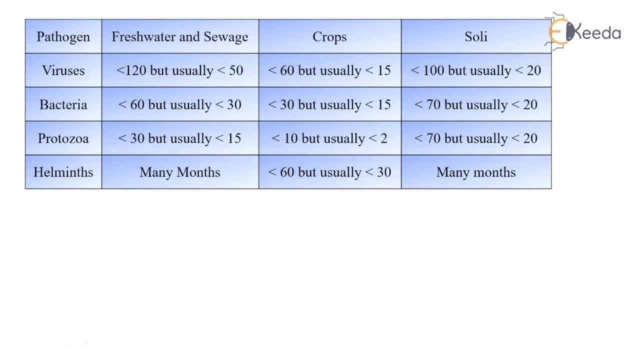 in the range of 50 to 120 minutes. Bacteria which are surviving in freshwater and sewage are present for the duration of 30 to 60 minutes. Protozoa are surviving in this wastewater are 15 to 30 minutes and helminths are surviving. 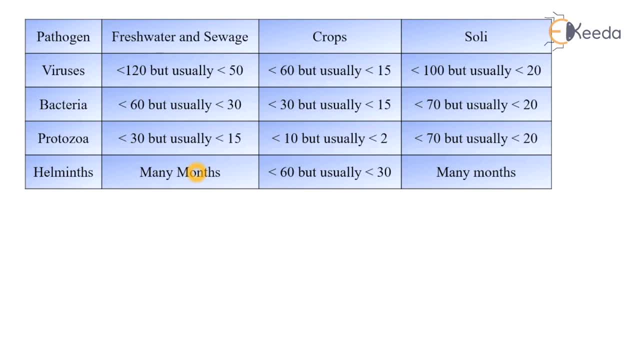 for the freshwater and sewage are many months. So similarly in crops these viruses or pathogens are surviving in crops. crop duration is for viruses is 15 to 60 minutes, bacteria is 15 to 30 minutes, protozoa is 2 to 10 minutes and helminths are usually survive for the longer time that is in. 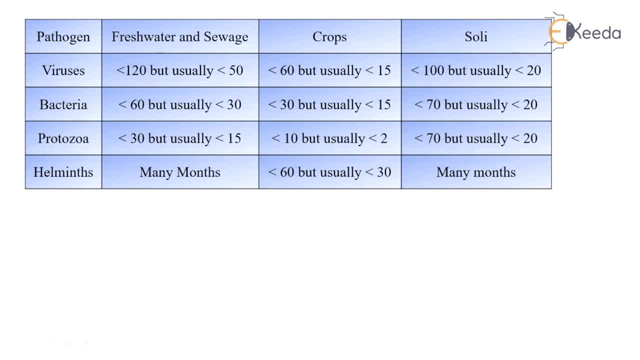 30 to 60 minutes and for soil for viruses are survival in between 20 to 100 minutes, bacteria are surviving in between 20 to 70 minutes, protozoa are surviving in between 20 to 70 minutes and again, helminths are surviving in it for the many months. 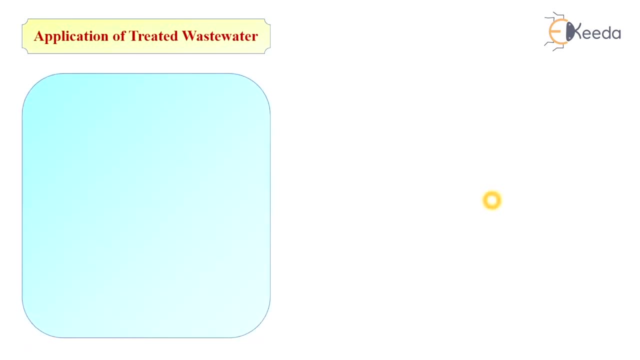 so what are the applications of treated wastewater, or we can call it as reusable water. so for the agricultural purpose or agricultural irrigation. so again, there are types like crop irrigation and commercial nurseries for landscape irrigation, so for parks, schoolyards, highway medians, golf courses. 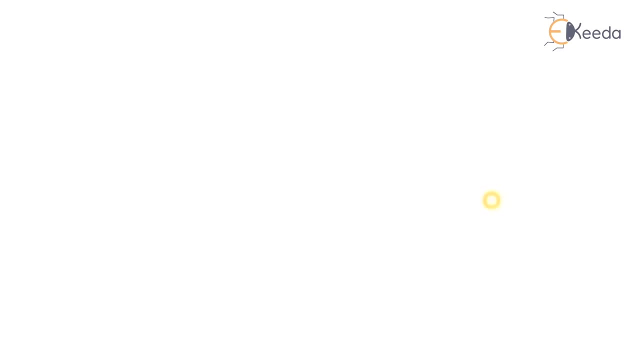 and for the agricultural purpose or agricultural irrigation. so again there are types like crop irrigation and commercial nurseries for landscape irrigation, cementaries, residential areas, etc. again, the reusable or treated water which is applicable for industrial recycling and reuse in form of cooling water boiler. 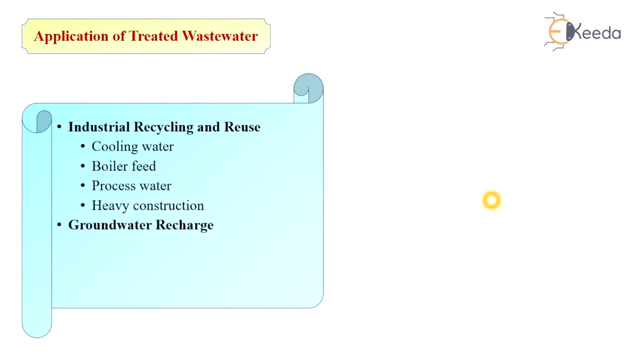 fill process water, heavy construction and for the groundwater recharge. the groundwater replenishment is required, the saltwater intrusion control is required and subsidence control is required again. there are recreational and environmental use of this treated wastewater in forms of lake and ponds, marsh enhancement, stream flow agmentation, fisheries and for non potable. 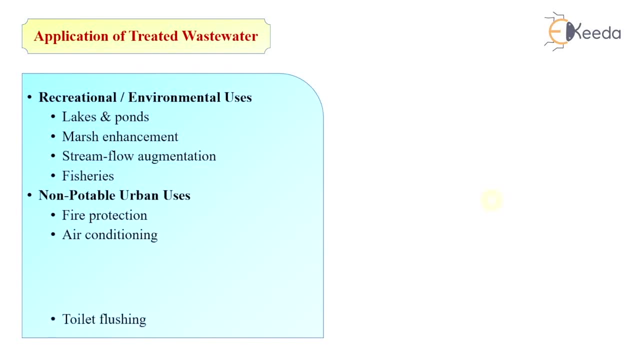 urban uses: the fire protection, air conditioning, toilet flushings for potable reuse, the blending in water supply reservoirs and pipe to pipe purification, so for the use of this treated wastewater. again, there are recreational and environmental use of this prepared water. in this case this is also known as pipe to pipe water supply. 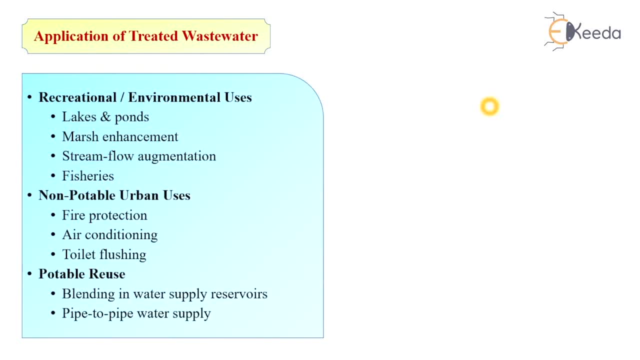 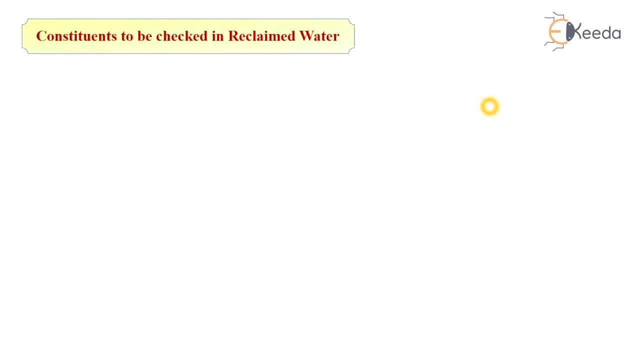 so for this reasons, we are having the reusable water for the purpose of this mentioned application or forms. and what are the constituents to be checked in, reusable water or reclaimed water? so there are different types of constituents or contents which are present in the re-recommendable. 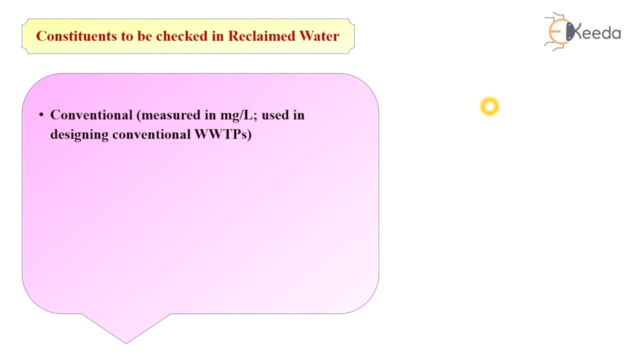 water or reusable water. so there are different types of constituents or contents which are present in the re-recommendable Water or Reusable water In terms of its standards. so for conventional use, in designing conventional wastewater treatment plant we are considering the parameters like total suspended solids, biochemical oxygen demand and chemical oxygen demand. total organic constituents, nitrogen contents in form of ammonia, phosphorus nitrate nitrites, phosphorus contents and 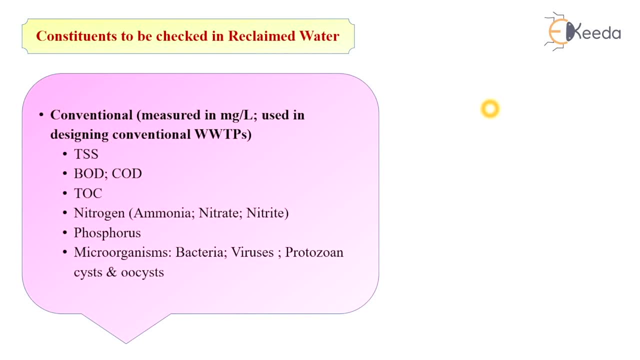 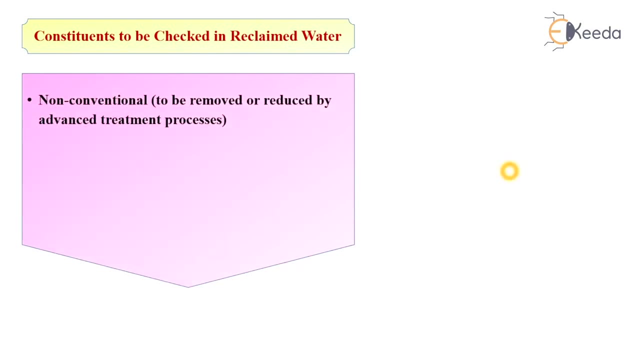 microorganisms in form of bacteria, viruses, protozoa, cysts, etc. So again for non-conventional use. we are using this reclaimed water for refractory organics, for volatile organic compounds, surfactants, metals, total dissolved solids, etc. 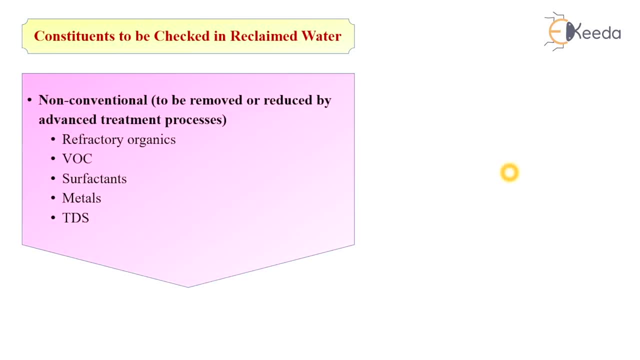 So for non-conventional use, conventional reusable water, we are considering these parameters. So next is problems associated with waste water reuse. What are the problems that we are facing during recyclable water? First is heavy elements For public health: the nervous system disorders, mutagenesis, tetraetogenesis, carcinogenesis For bioaccumulation food chain. 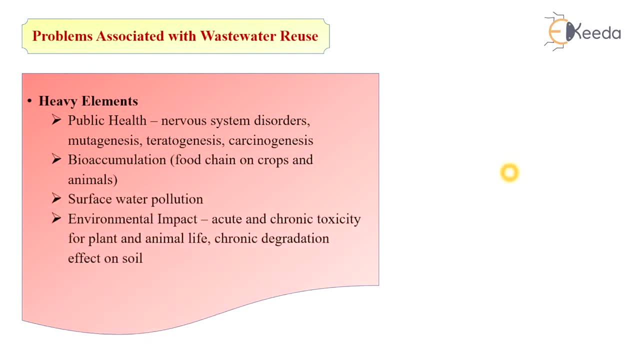 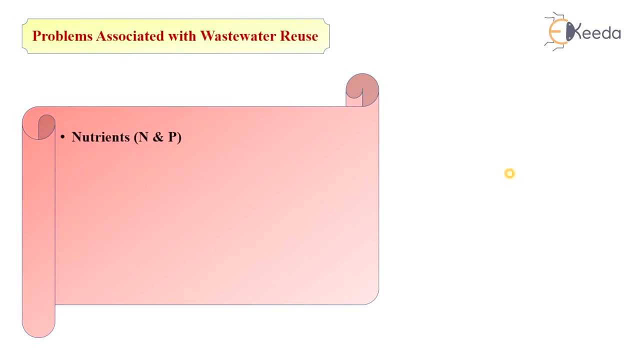 on crops and animals For surface water pollution. For environmental impact like acute and chronic toxicity for plant and animal life, Chronic degradation effect on soil For nutrients like nitrogen and phosphorus. the public health in public health. if this limit of this constituents is exceeded, then the childhoods of animals and animals will be affected. So for the use. 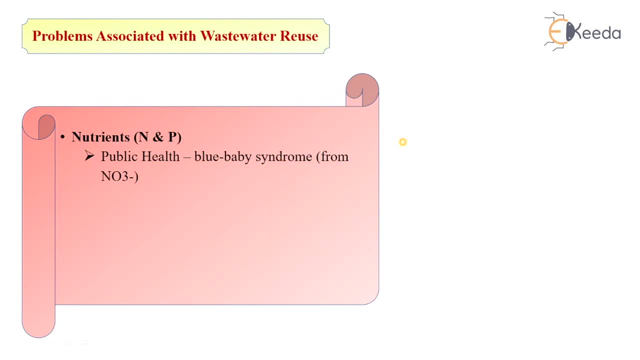 of bioaccumulation products. we are considering these problems. So what are the problems that or childrens are facing? problems or disease like due baby syndromes, the infiltration into potable water supplies, the environmental health, the eutrophication or crop yield effect. 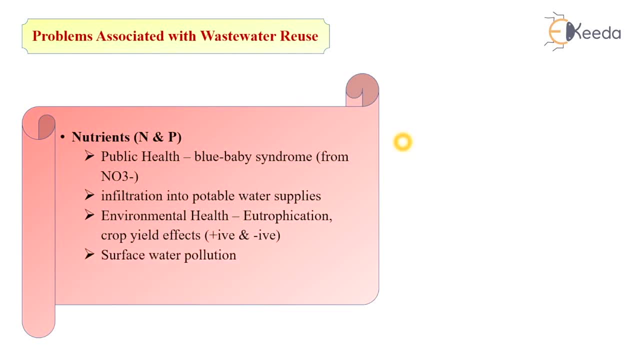 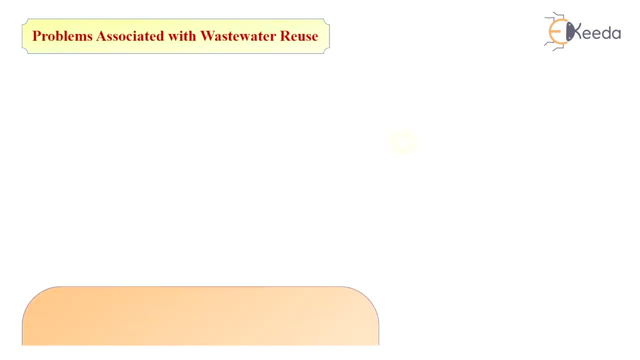 are happening while exceeding the nutrients contents in waste water. surface water pollution is occurs and irrigation practices Again the dissolved solid contents are exceeded to form the salinity. the environmental health is affected, the induced problems for the crop, seed selection and quantity accumulation. 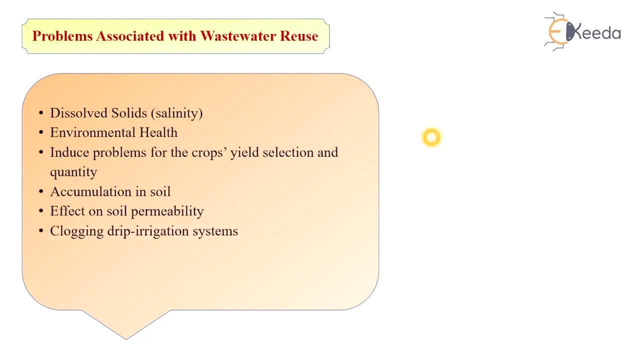 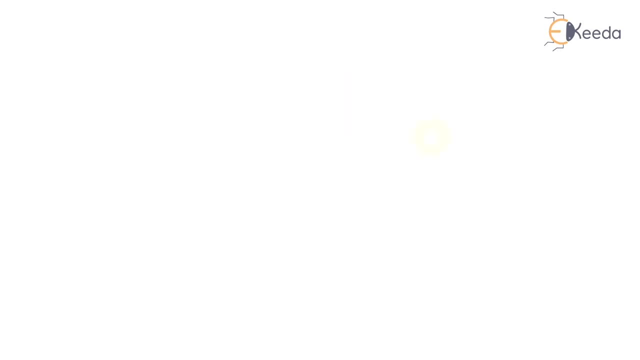 in soil, effect on soil permeability, clogging, drip irrigation system, emerging pollutants, public health. So these are some problems that we are facing. While the constituents in the treated sewage is exceeded, again, some groundwater contamination is there when the constituents are, or parameters are, greater in this reusable water, like nitrate. 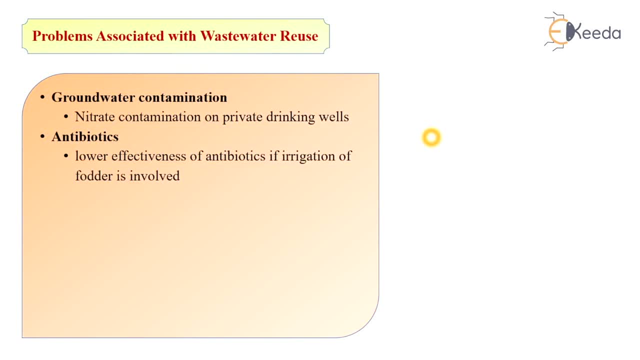 contamination on private drinking wells. the antibiotics: the lower the effectiveness of antibiotics if irrigation of fodder is involved. odour the public health of neighbouring communities. aesthetic concern reduces land values. The concern with industrial processes like scaling, corrosion, biological growth and 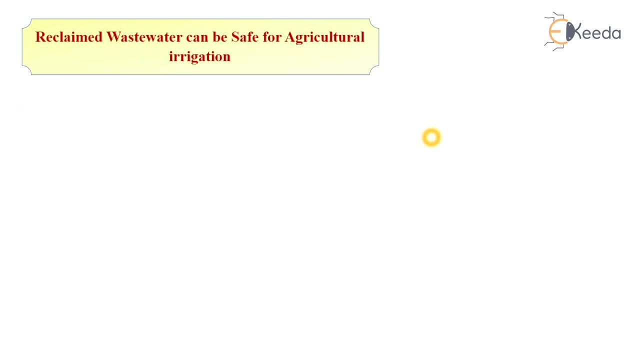 fouling, etc. So the reclaimed waste water can be safe for agricultural irrigation. How It reduce the pathogen level. avoid the direct contact of crop with reclaimed waste water. restrict the type of crop irrigated. Different types of irrigation methods can be used. 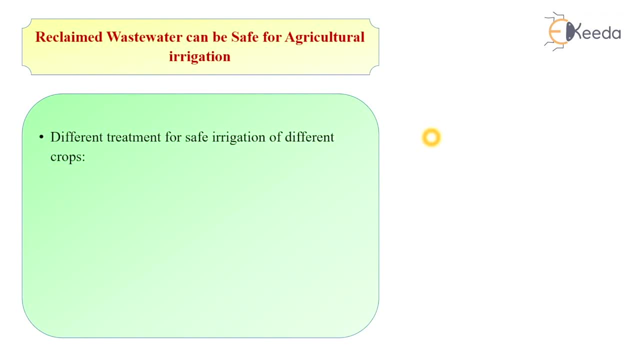 Different types of irrigation methods can be used. Different types of irrigation methods can be used, That is, the cloth cage or floor treatment, soil priming. We are providinglavlan treatment for safe irrigation of different crops, For example for tree nurseries, pasture, industrial crops. 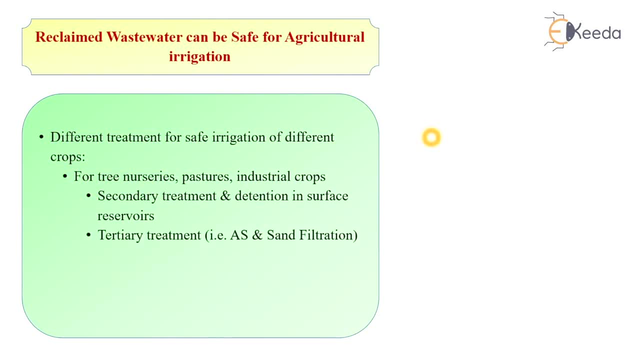 Secondary treatment and detention in surface reservoir are provided. sometimes we are providing the tertiary treatments like sand filtration or activated sludge For edible crops. we are providing the tertiary treatment followed by the soil aquifer treatment. So there are some guidelines for soil localization. 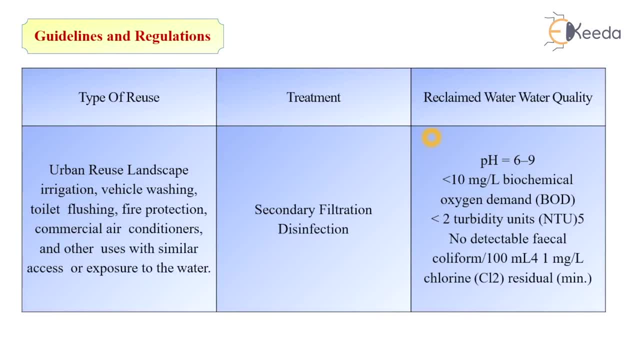 In the soil. soil for irrigation is required, It is preferred that water nutritional, intimate contact is maintained. guidelines for the discharge standards, for example, when we are using the treated waste water or reusable water for the urban purposes, for the purpose of landscape irrigation, vehicle washing, toilet flushing, fire protection, commercial air conditioner and other uses. 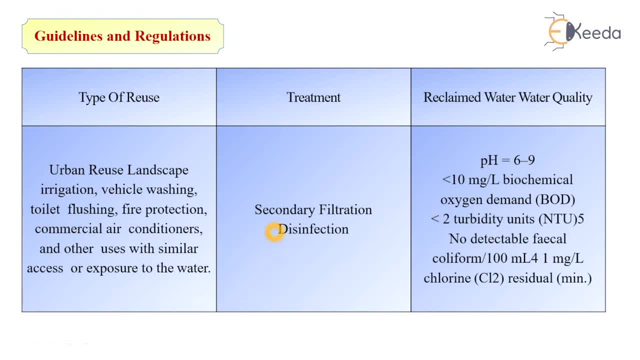 we are providing the secondary filtration or disinfection in form of treatment and the discharge standards for the use of these purposes. the parameters considering and its discharge values are as follows. so if the treated sewage has the pH value of in between 6 to 9, it has 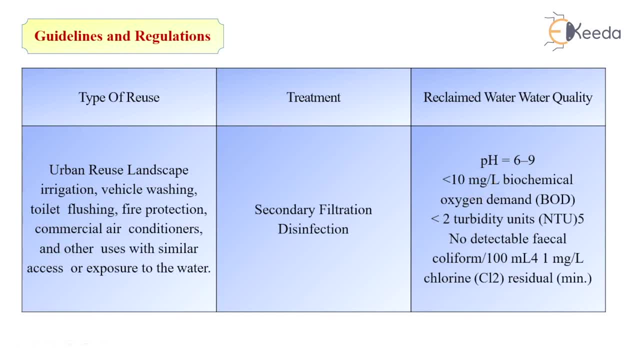 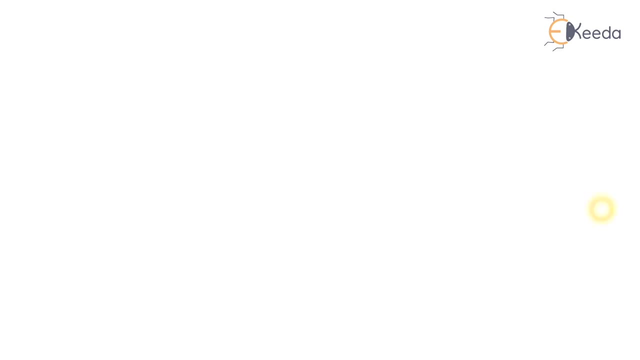 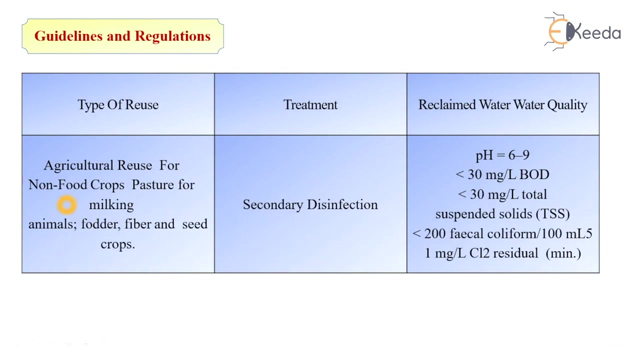 free from CO2 or fecal polyform or bacterium chlorine residues. so while we are using this treated water for the purpose of agricultural, for non-food crop pasture for milking animals, fodder fibers and seed crops, the secondary disinfection is provided and the parameters that we have considered for these treatments. 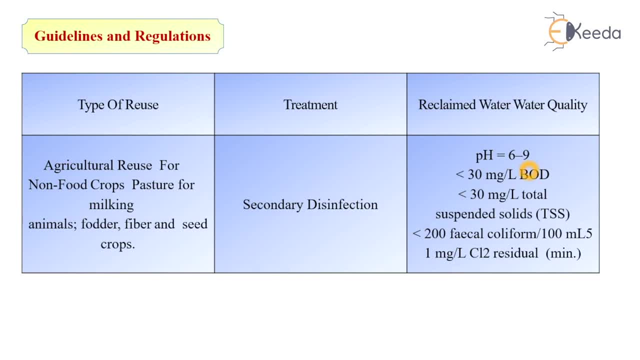 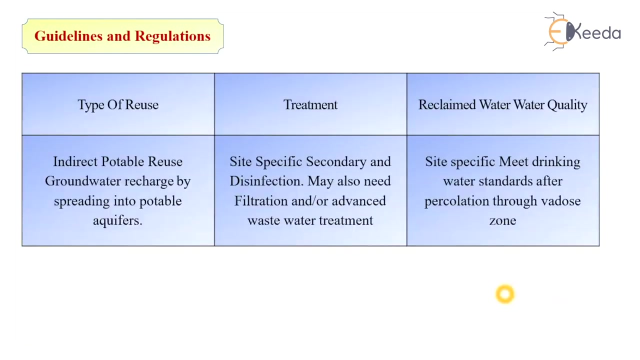 are pH values in between 6 to 9, the BOD is in the range less than 30 mg per liter, the total suspended solids are less than 30 mg per liter and the fecal polyforms are less than 200 per 100 ml of chlorine residues. again, when we are using this treated water for the 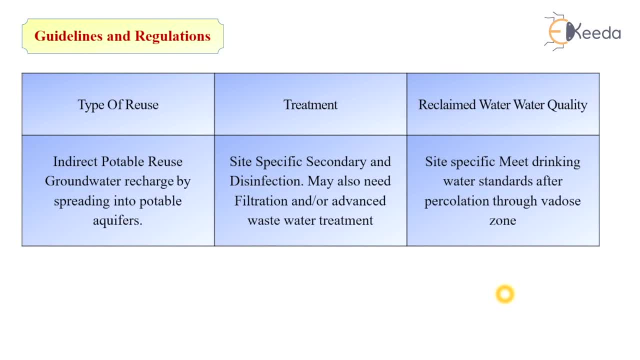 purpose of indirect potable reuse, groundwater recharge by spreading into the potable aquifer. we are providing the treatment, such as site specific, secondary and disinfection. we are providing the treatment, such as the treatment, such as the chemical reaction may also need filtration and or advance wastewater treatments. for the water quality parameter: the site specific. 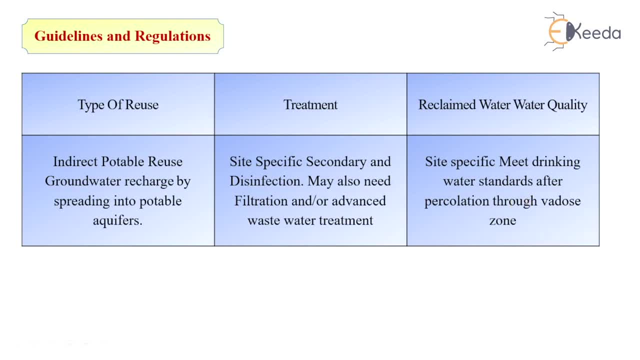 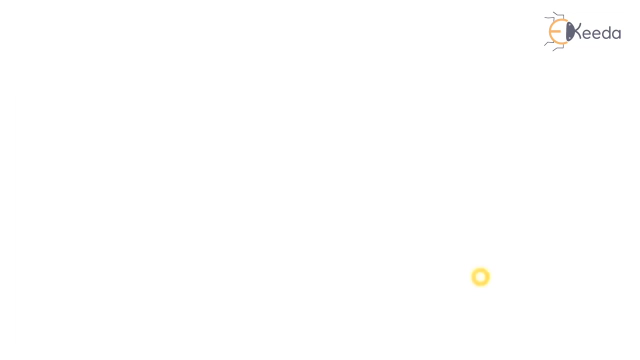 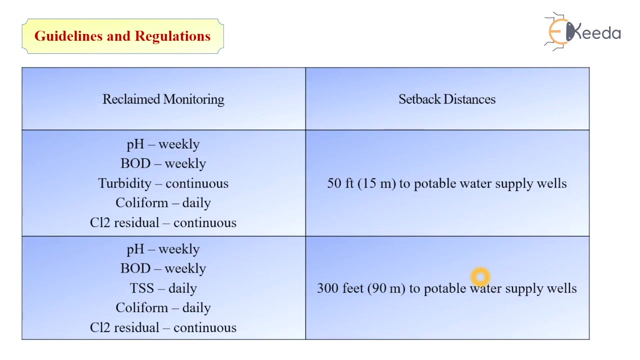 meet drinking water standards after percolating through the water zone, because one of the source of drinking that is groundwater source. so many times we are using this groundwater for the drinking purpose. so for the standards we are providing for the drinking water, qualities are expected here for the treated water. so the reclaim monitoring parameters. so we are observing. 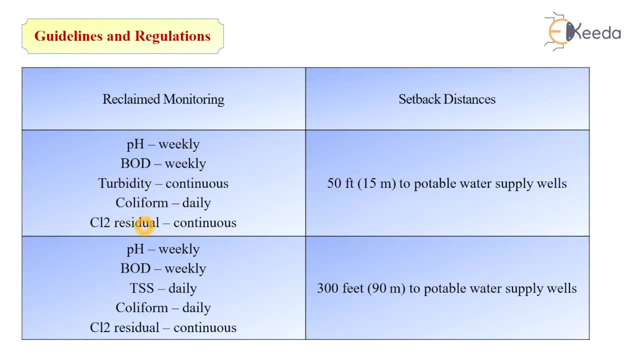 or analyzing this ph bod turbidity polyform and chlorine residuals values on either daily, weekly or continuous basis. the setback distance is 50, 50 feet or 15 meter to portable water supply. well for analyzing ph bod weekly and tss polyform daily, the 300 feet or 90 meter. 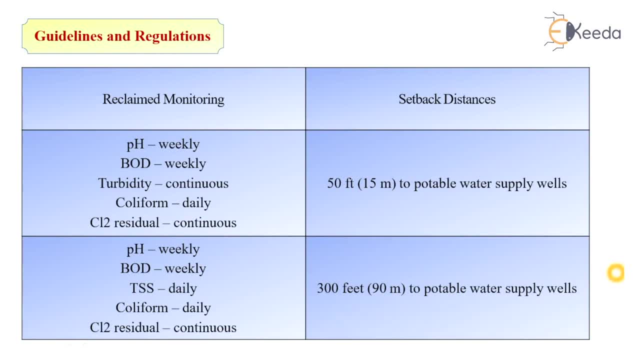 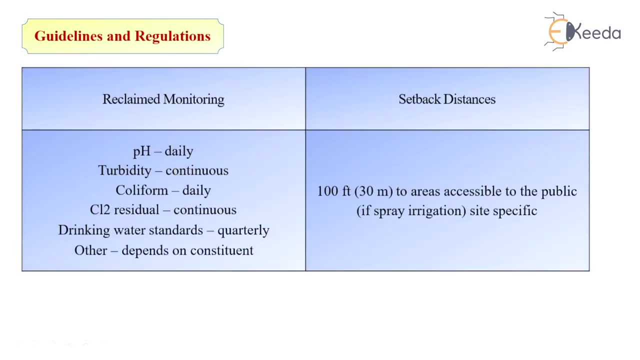 setback distance is provided to portable water supply. well, again, the ph or turbidity polyform which are analyzing on daily basis, and chlorine residue is continuous basis and drinking water standards are quarterly basis. so we are analyzing the ph bod weekly and tss polyform daily, the 300 feet or 90 meter setback. 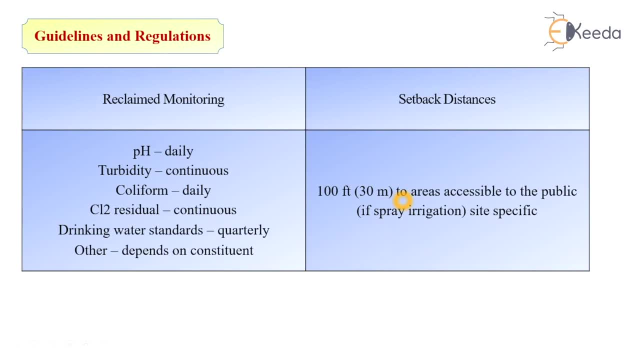 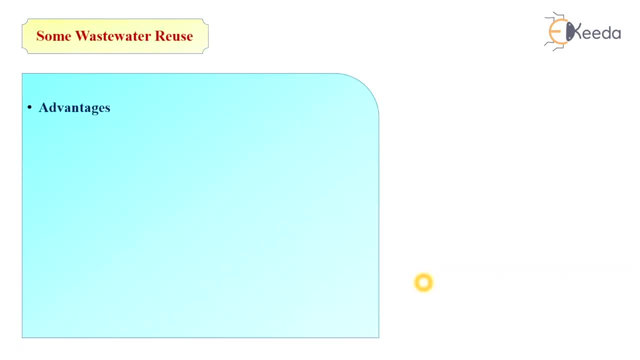 the 100 feet or 30 meter setback distance to provide it for the areas accessible to the public site specified. so some of the advantages of this treated or reusable waters. this technology reduces the demand of portable sources of fresh water. it may reduce the need for large wastewater. 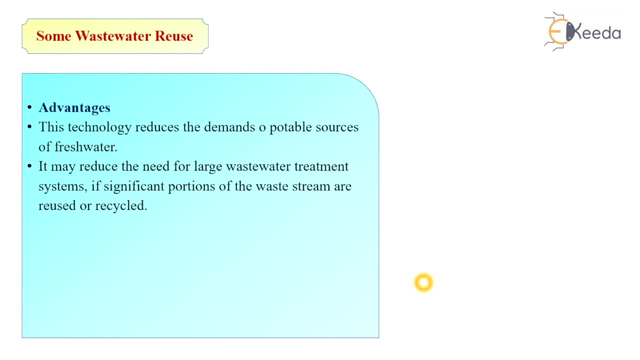 treatment system. if significant portions of the waste stream are reused or recycled, the technology may diminish the volume of wastewater discharge, resulting in the beneficial impact on the aquatic environment. the capital cost are low to medium for most system and the recoverable in the very short time. this excuse the systems designed for direct reuse of sewage water. 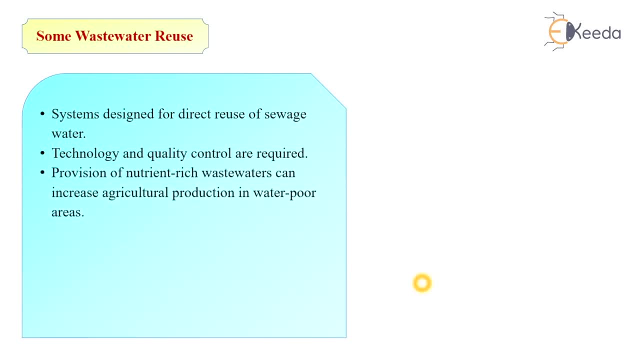 technology and quality control are required. provision of nutrients rich wastewater can increase the agricultural production in water poor areas, pollution of river and groundwater may be reduced. the operation and maintenance are relatively simple, except in direct reuse system. where more extensive and there are some disadvantages, like if implemented on the large scale, the revenue to water supply and wastewater utility may fall as the 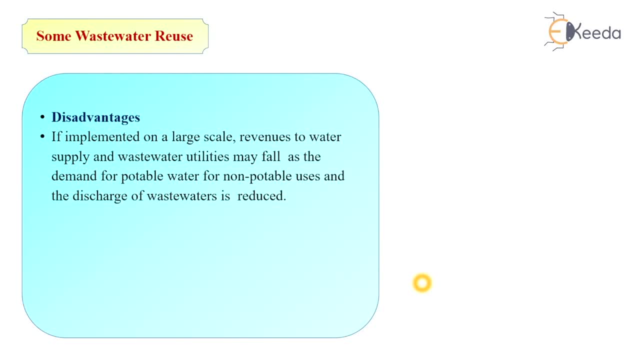 and there are some disadvantages, like: if implemented on the large scale, the revenue to water supply and wastewater utility may fall as the demand for portable water for non potable uses and the discharge of wastewater is reduced. reuse of wastewater may be seasonal in nature, resulting in the overloading of treatment and disposal facilities during the rainy seasons. if the wet season is of long duration and or high intensity, the seasonal discharge of the raw wastewater may occur. 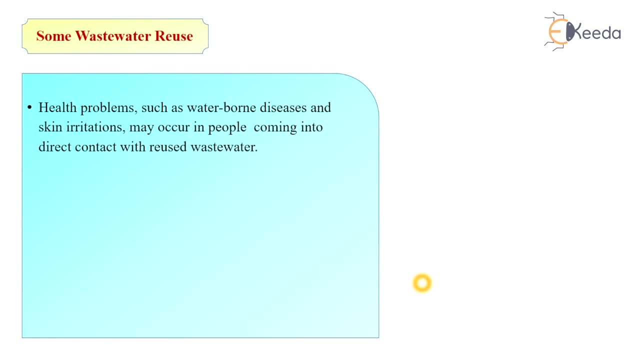 again. again. according to, health problems such as water-borne diseases and skin irritation may occur in people coming into direct contact with reused wastewater. Gases such as sulfuric acid produced during the treatment process can result in chronic health problems. In some cases, reuse of wastewater is not economically feasible because of the requirement. 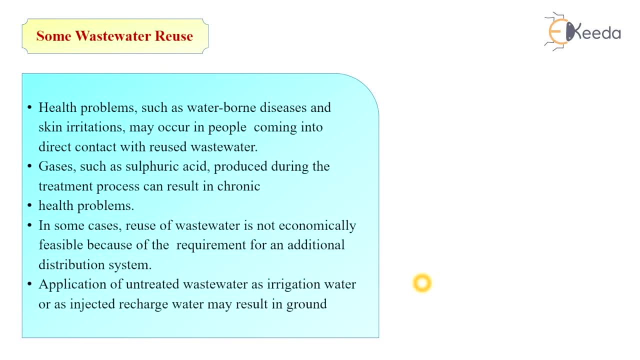 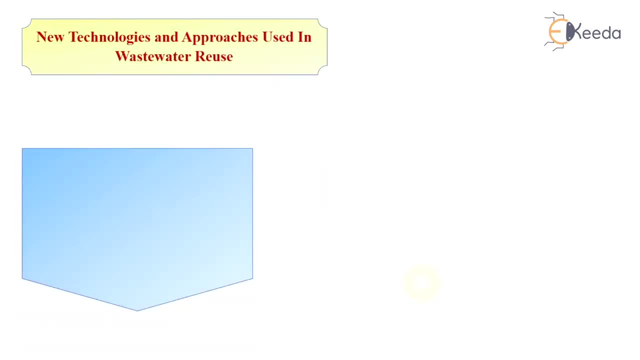 of the additional distribution system and application of untreated wastewater as irrigation water or as injected recharge water may result in ground pollution. Some of the new technologies and approaches used in the wastewater reuse, like membrane filtration, nanotechnology, microbial fuel cells, natural treatment system and urine. 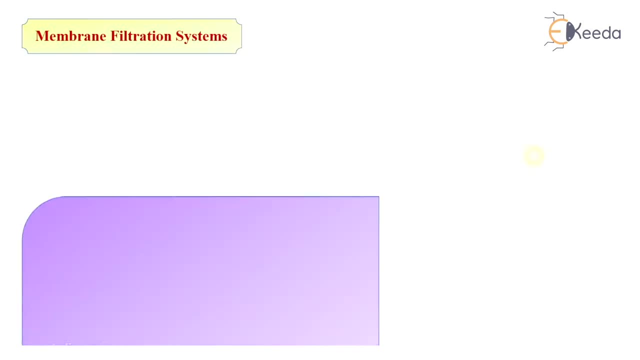 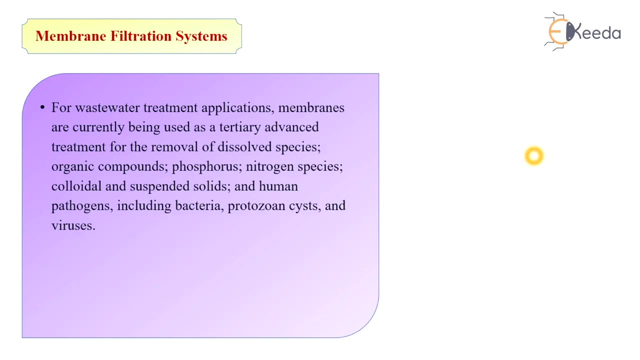 separating toilets. So first is Membrane Filtration System For wastewater treatment application. the membranes are currently being used as a tertiary advanced treatment for removal of dissolved species, organic compounds, phosphorus, nitrogen species, polydyl and suspended solutes and human pathogens, including bacteria protozoa. 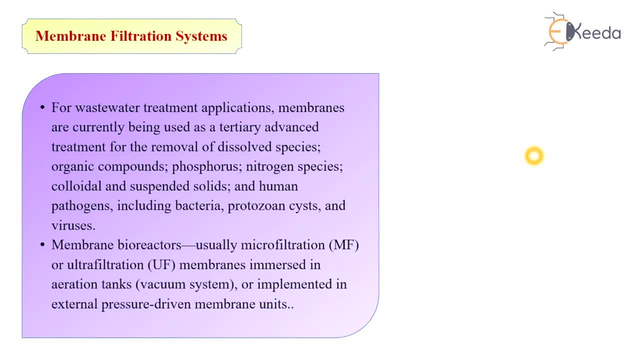 cysts and viruses. The membrane bioreactors: usually microfiltration or ultrafiltration membranes immersed in aeration tanks or implemented in external filters are used for filtration purposes. The membrane bioreactors: usually microfiltration or ultrafiltration membranes immersed in aeration. 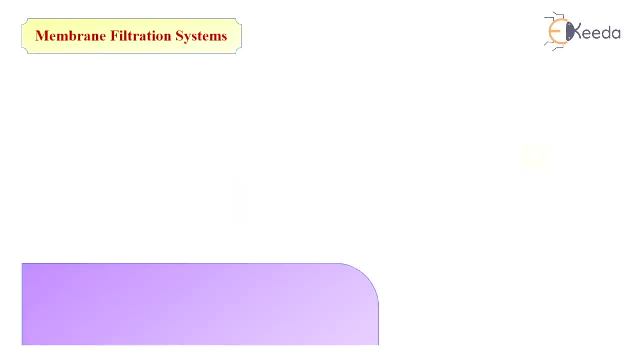 tanks or implemented in external filters are used for filtration purposes A low pressure membrane such as microfiltration or ultrafiltration membranes, either as pressure system or an immersed system providing a higher degree of suspended solids. The ultrafiltration membranes are effective for virus removal. 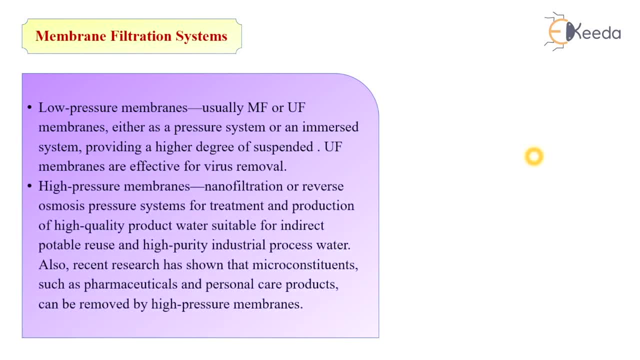 The high pressure membranes, such as nanofiltration or reverse osmosis pressure system, for treatment and production of high quality product waters suitable for illegal spillage or in which flower bed can be taken out, suitable for indirect potable reuse and high-purity industrial process water. 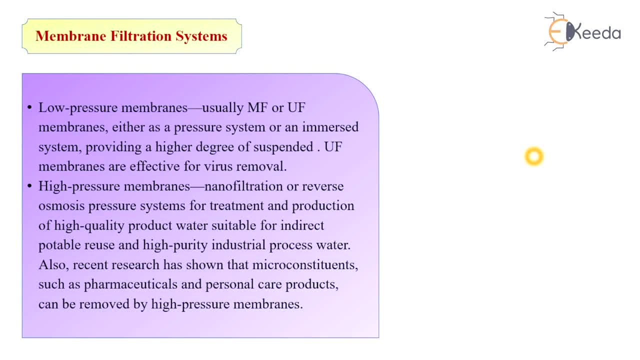 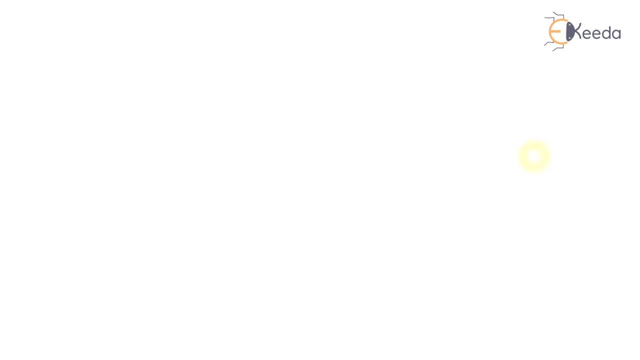 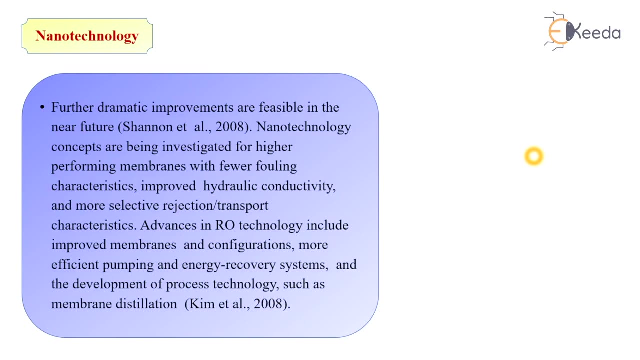 Also, the recent research has shown that the micro-constituents, such as pharmaceuticals and personal care products, can be removed by high-pressure membranes. So in nanotechnology, the further dramatic improvements are feasible in the near future. The nanotechnology concepts are being investigated for higher-performing membranes. 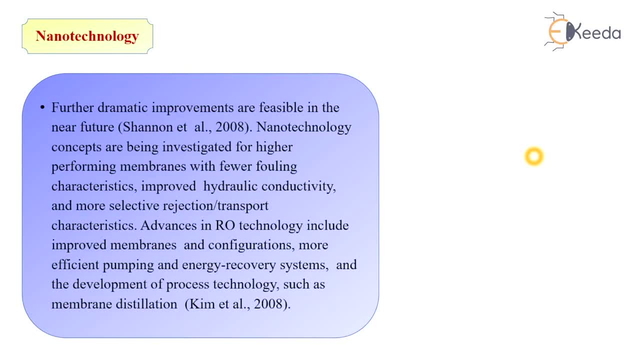 with fever-fouling characteristics, improved hydraulic conductivity and more selective rejection or transport characteristics. The advance in reverse osmosis technology includes the improved membrane and configuration, more efficient pumping and energy recovery system and the development of process technologies such as membrane distillation. 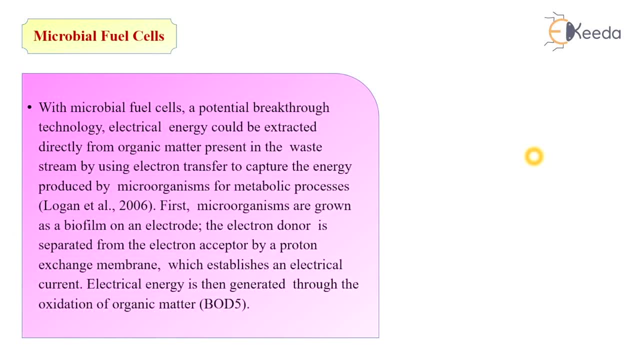 The microfuel cells, with microbial fuel cells, a potential for the development of a new energy recovery system. and the development of a new energy recovery system. The electrical energy could be extracted directly from the organic matter present in the waste system by using the electron transfer to capture the energy produced by microorganisms for metabolic processes. 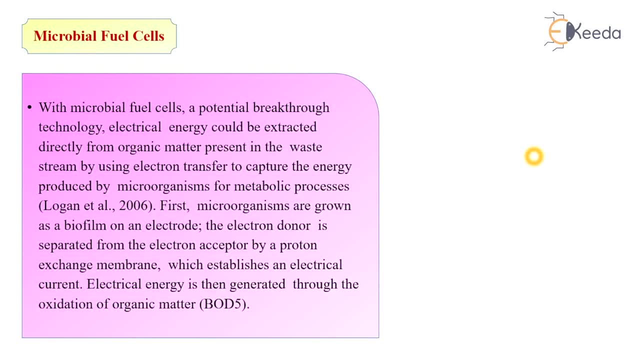 First, microorganisms are grown as a biofilm on an electrodes. The electron donor is separated from the electron acceptor by a portion exchange membrane which establish an electrical current. The electron donor is separated from the electron acceptor by a portion exchange membrane. 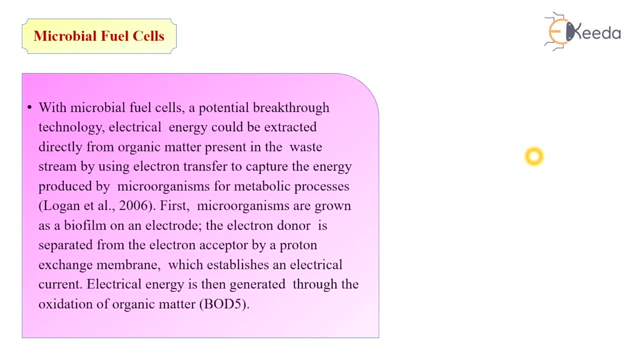 which carries in electrical energy by constantly passing through the Oxygen of an ion to the diffusion circuit. at That point it looks likeอмаix384Ω Stern. It's a steam fer. ESO-Aежду Ice diesexion робото. thirteen ginseng студium. 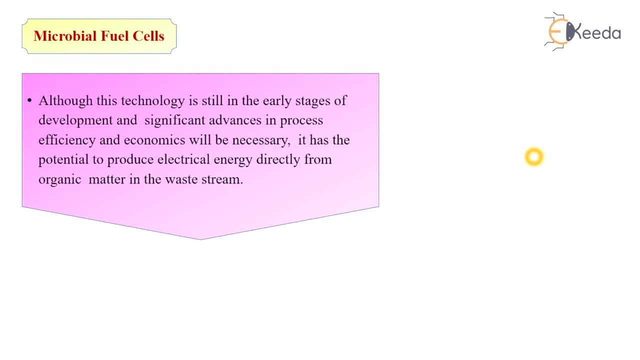 Although this technology is still in the early stages of development and significant advances in process efficiency and economics will be necessary, It has the potential to produce the electrical energy directly from the organic matter in the waste tool, so it is a very important application of the reuse of. 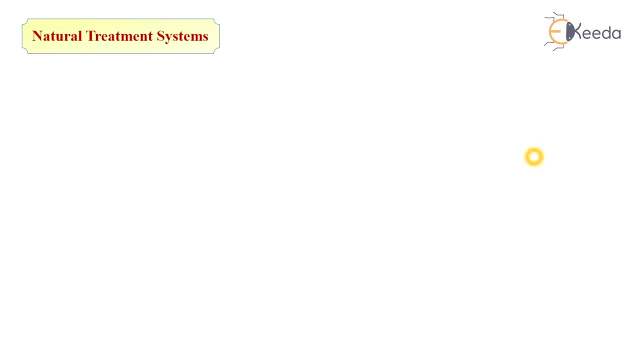 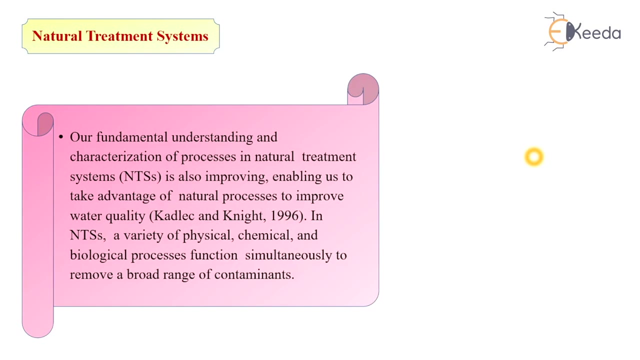 wastewater or sewage in some of the natural treatment system. like our fundamental, understanding and characterization of process in natural treatment system is also improving, enabling us to take advantage of natural processes to improve the water quality. in natural treatment system, the variety of physical, chemical and biological processes functions simultaneously to 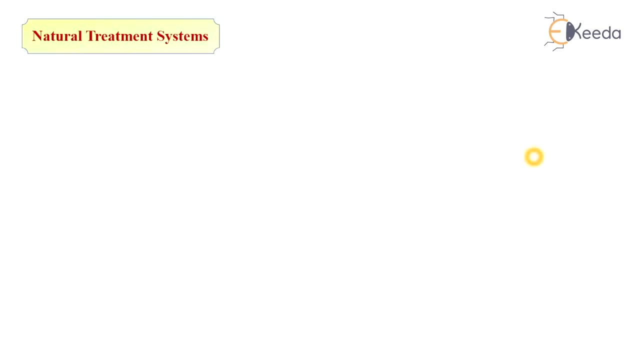 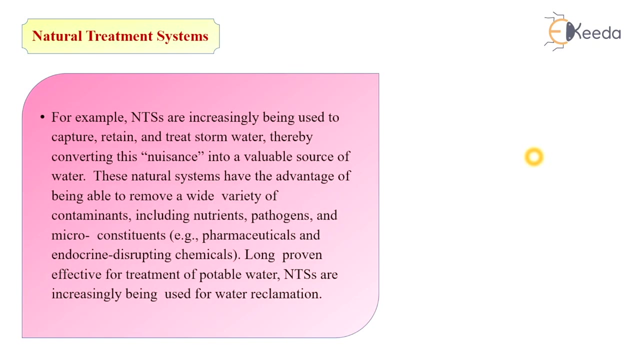 remove the broad range of contaminants. for example, in natural treatment system are increasingly being used to capture, retain and treat storm water, thereby converting this nuisance into the valuable source of water. these natural system have the advantage of being able to remove a wide variety of contaminants, including nutrients, pathogens and 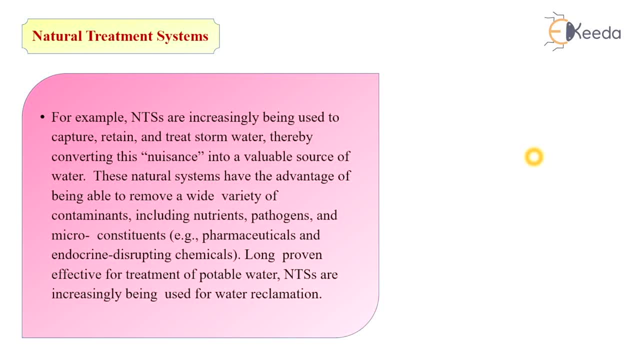 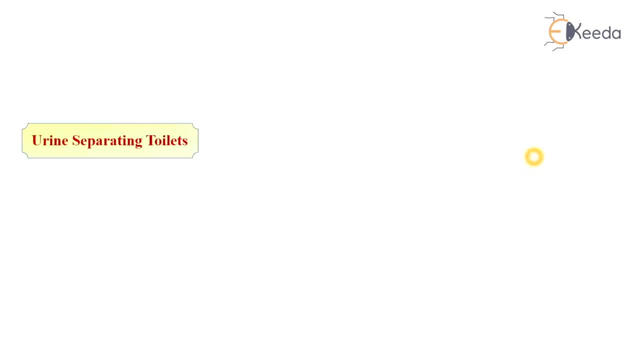 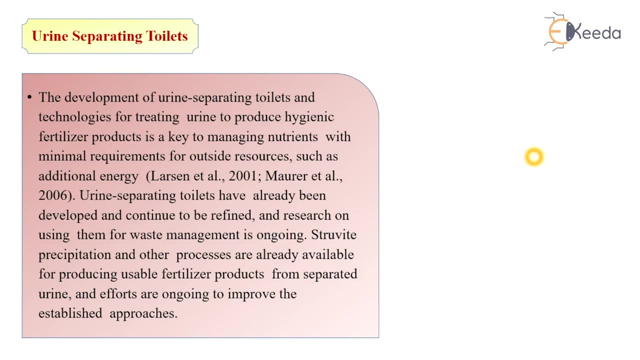 micro constituents long-term effective for treatment of potable water. the natural treatment systems are increasingly being used for water reclamation. then the urine separating toilets. the development of urine separating toilets or technologies for treating urine to produce hygienic fertilizer product is a key to managing nutrients with minimal requirement of outside resources such as. 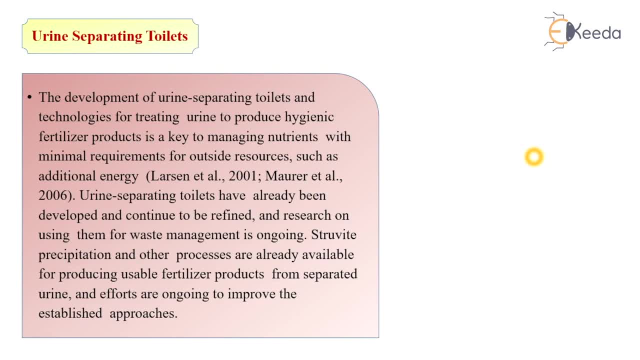 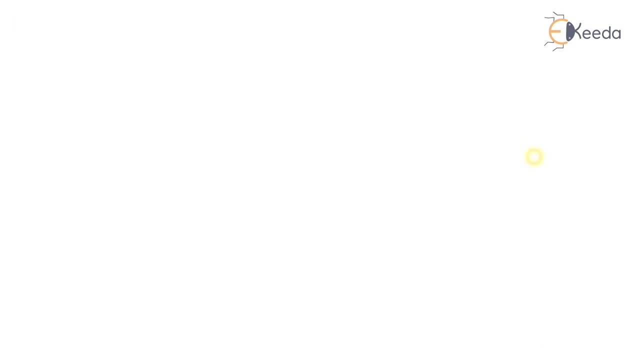 additional energy. urine separating toilets have already been developed and continue to be refined, and research on using them. of waste management is ongoing. Servai, precipitation and other processes are already available for producing the usable fertilizer products from separated Europe, and efforts are ongoing to improve the established approaches. Then these are some case studies, just for your. 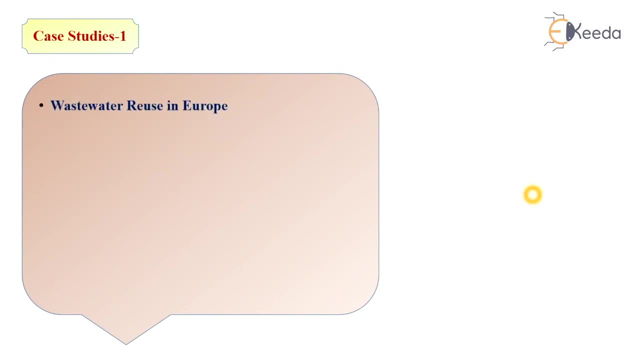 understanding So in other countries, how they are reclaim this sewage or waste water. So in European countries, the last two decades has witnessed growing water stress, both in terms of water scarcity and quality deterioration, which has promotes many municipalities to look for the more efficient use of water resources, including more widespread acceptance of 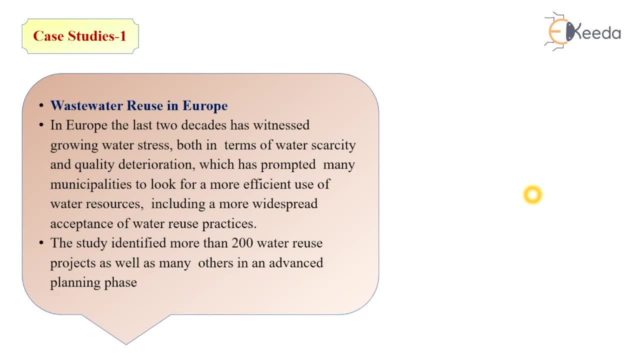 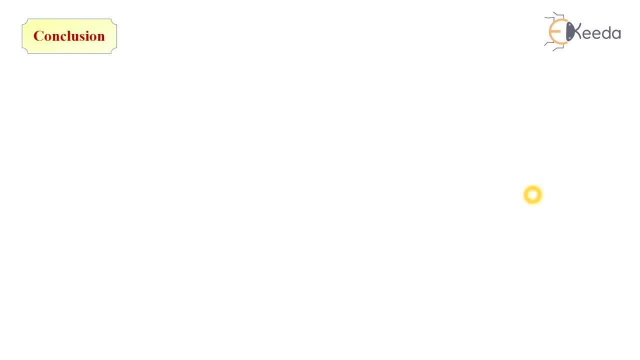 water reuse practices. So the study identified more than 200 water reuse projects, as well as many other in an advance planning course. So conclusion from this case study is the almost all medium and large scale schemes have been designed as add on technology to. 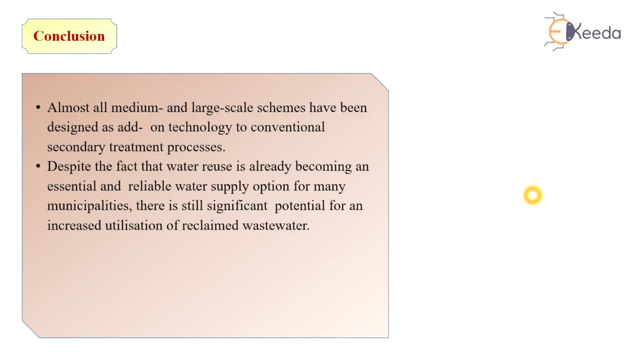 conventional secondary treatment processes, Despite the fact that water reuse is already becoming an essential and required process. So the study identified more than 200 water reuse projects in the future. This reason alone, seeing an increase in the water use market- happens because the way of administration of system at so some later stages is 케. 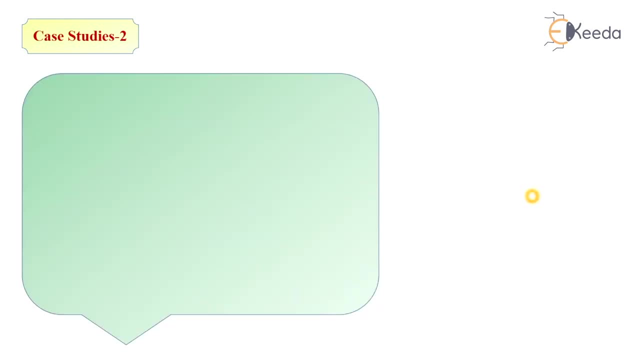 in the land. In second case study, the wastewater quality and reuse is irrigation in Kuwait using microfiltration technology in treatment. So microfiltration unit has been tested in Kuwait Institute for scientific research to treat the secondary wastewater effluent from Rika Wastewater Treatment Plant. 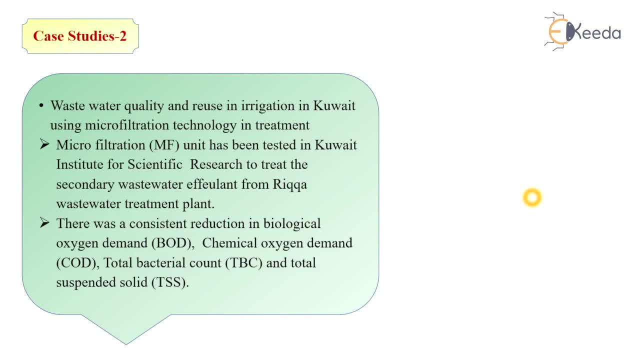 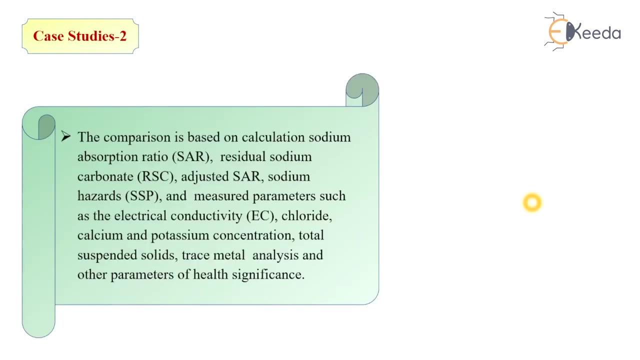 There was a constituent reduction in biological oxygen demand, chemical oxygen demand, total bacteriological count and total suspended solids. So the comparison is based on conclusion: sodium adsorption ratio, the residual sodium carbonate, the adjusted SAR, the sodium hazardous and measured parameters such as the electrophoresis. 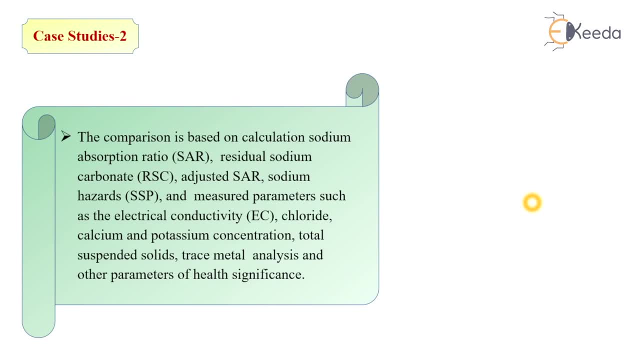 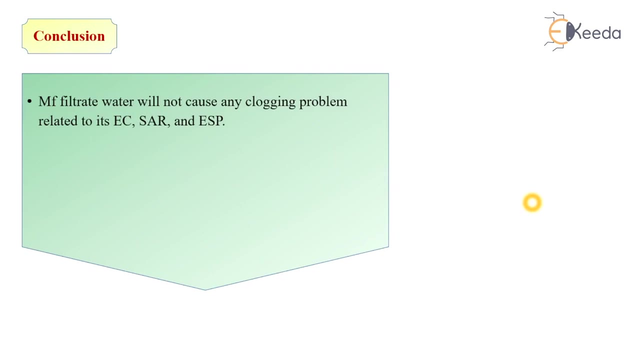 Electrical conductivity, chloride, calcium and potassium concentration, total suspended solids, trace metal analysis and other parameters of health significance. So conclusion from this: the microfiltration water will not cause any clogging problem related to other technology. Only the chloride potential might causes a moderate potential problem. 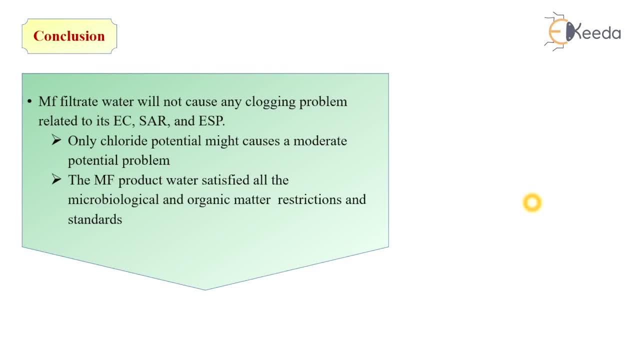 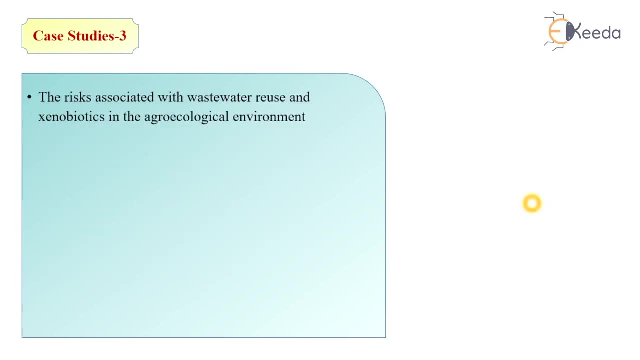 The microfiltration product water Satisfied all the microbiological and organic matter restrictions and standards. So another the again the different case study: the risk associated with wastewater use and xenobiotics in the aerocological environment, agroecological environment. 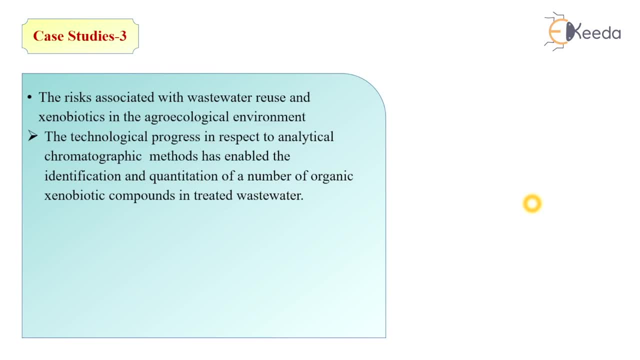 The technological progress in respect to analytical chromatographic method has enabled the identification and quantification of number of organic matter. It is also widely accepted that the currently applied treatment processes for urban wastewater abatement fail to completely remove such a contaminant, and this leads to their subsequent release in the terrestrial and aquatic environment through the disposal and reuse application. 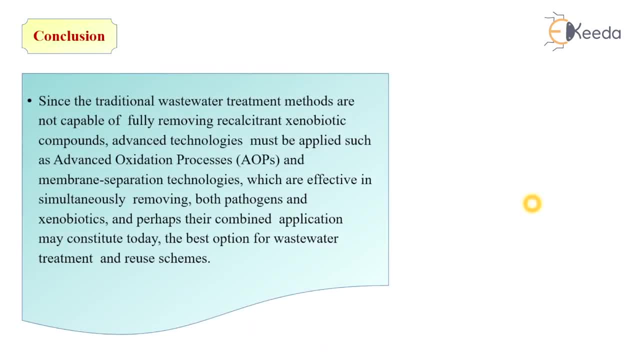 So conclusion from this case study is: Since the traditional wastewater treatment method are not capable of fully removing Reclamation zeobiotic compounds, the advanced technology must be applied, such as advanced oxidation process and membrane separation technologies, which are effective in simultaneous removing both the pathogens and xenobiotics, and perhaps their combined application may constitute today the best option for wastewater treatment and reuse scheme. Subtitles by the Amaraorg community.